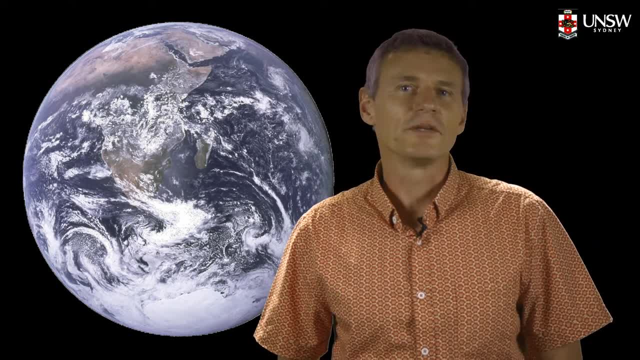 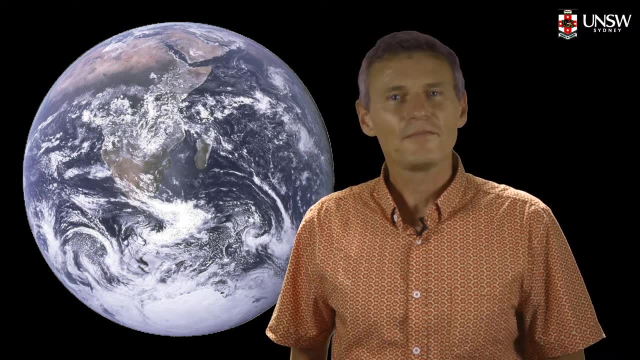 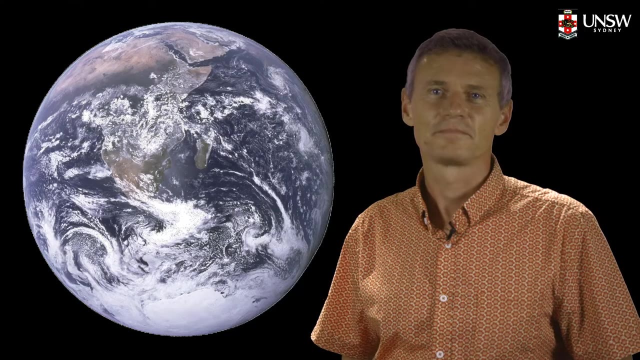 It was taken on one of the Apollo missions in the early 1970s And when you think about it, that's actually not very long ago. Only 50 years ago, no human being had ever seen planet Earth from this perspective. At that time, no one thought that one day. 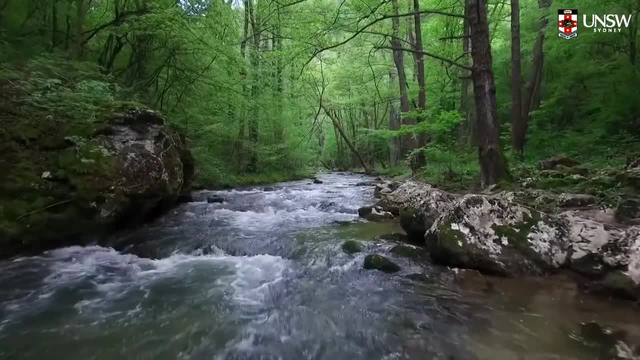 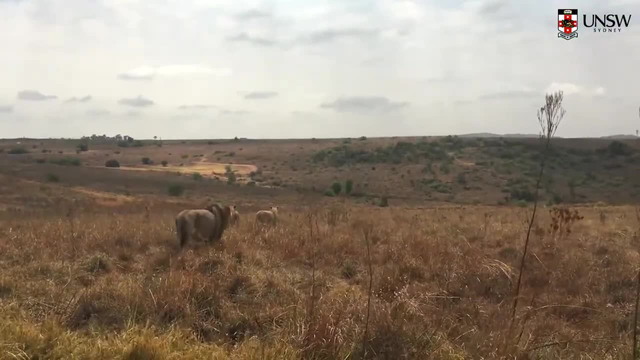 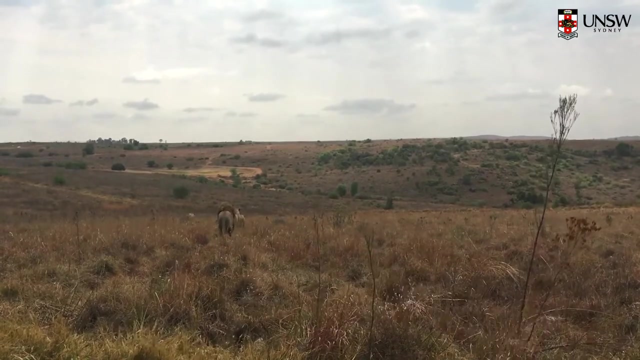 only 50 years later, there might be a problem with life on this planet. This week will all be about sustainability. but what actually is sustainability? If someone asked you this question, you can answer with a simple statement. You can just say: sustainability is. 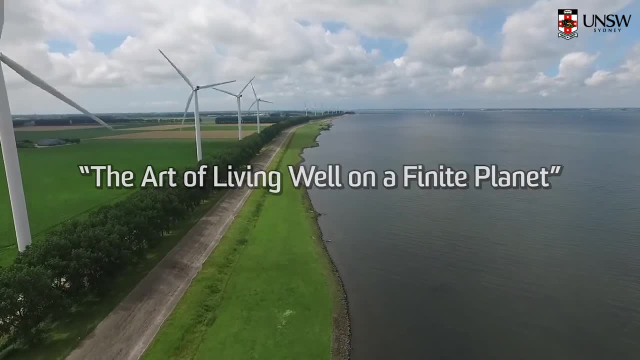 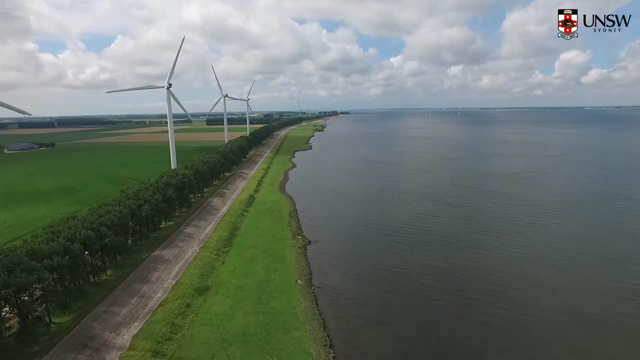 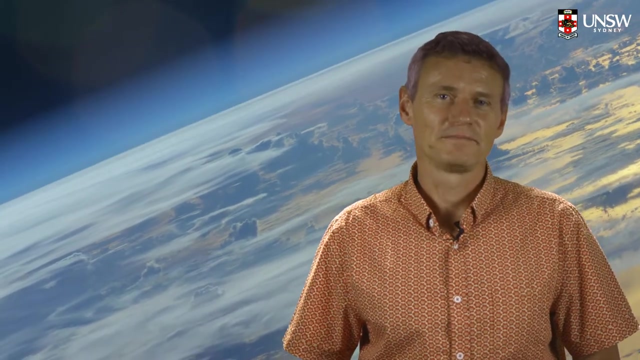 the art of living well on a finite planet Too easy. Of course, there is much, much more behind this statement, And this is what we will explore this week. So let's start with a finite planet. This one planet, Earth, is all we've got to live on. The more people we are, the more we. 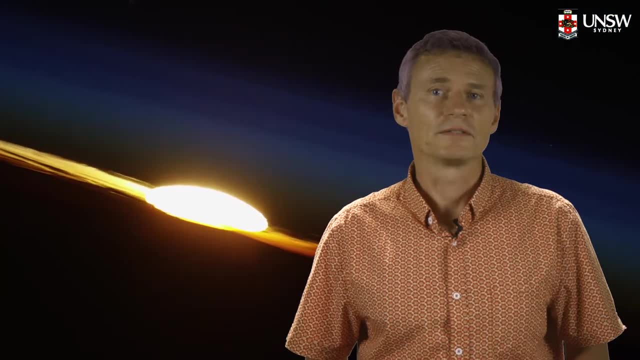 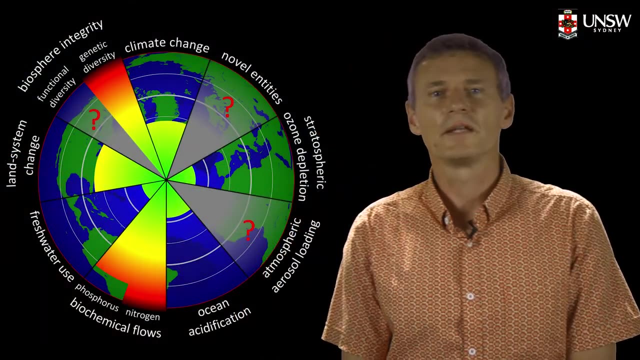 produce and consume, the more we put this Earth under system, under pressure. Scientists have worked out that human influence has now irreversibly changed function of human life. But what about structural change? And how can we create a more sustainable human society? And from this we will be looking at the world now As the world changes, and also in a more 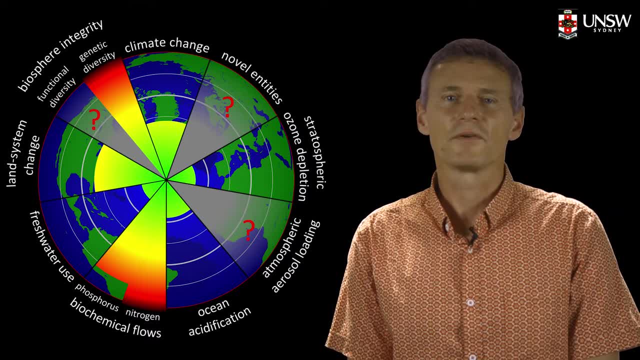 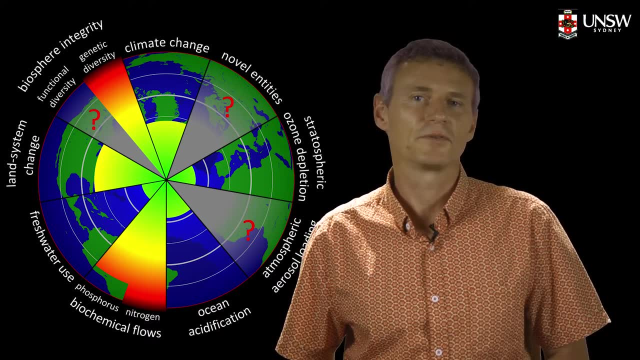 progressive way we will be looking at the world. as yet The world is changing. We will be of the system. In other words, we have already transgressed some of the planetary boundaries that define a safe operating space for humanity. You will. 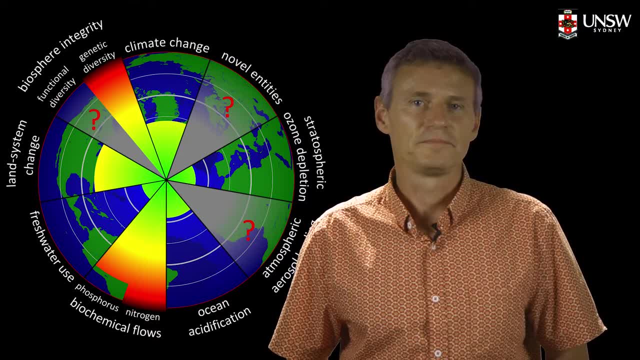 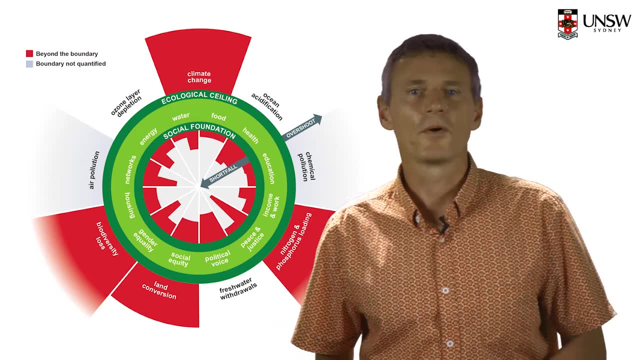 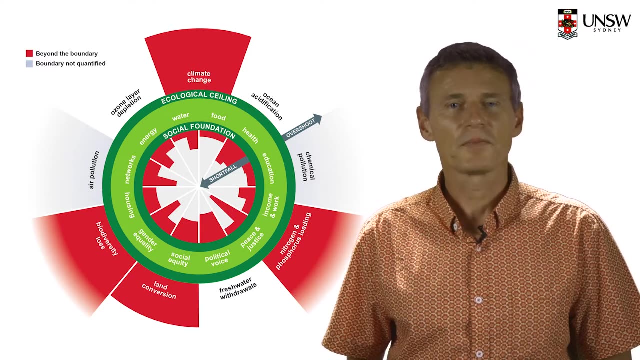 learn what these boundaries are and why they matter. But it is not only about the natural environment. As you will see this week, both society and economy are two other important domains for sustainability. As with planetary boundaries, we can actually define social boundaries, or you could call the minimum. 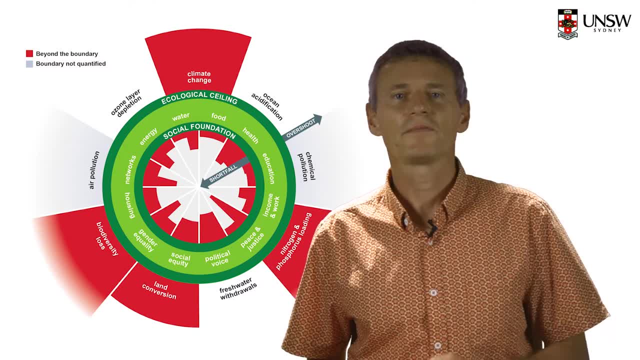 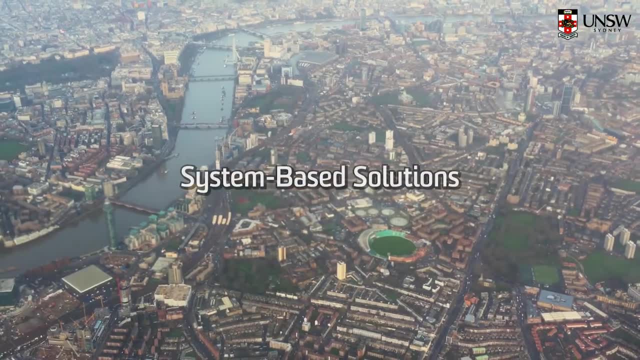 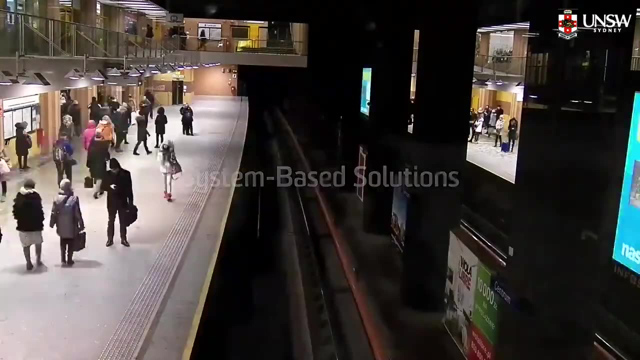 social and economic standards that we have to achieve or maintain in order to be truly sustainable. You will learn about principles for sustainability and how they can be applied to engineering. More than ever, engineers need to find holistic and sustainable solutions to their problems. You will learn about the